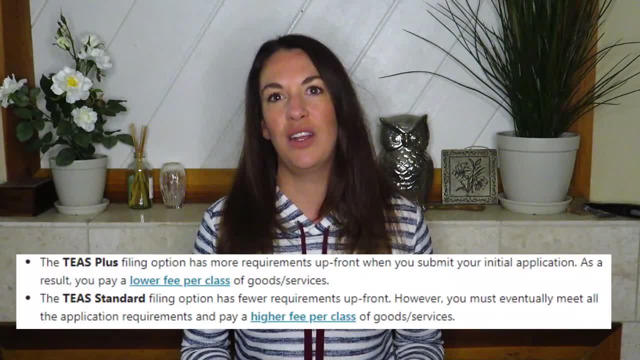 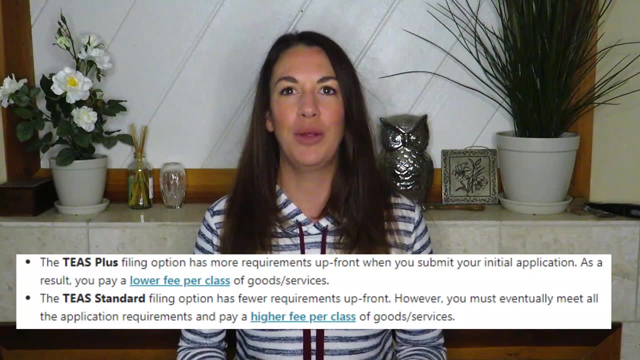 TEAS Plus and TEAS Standard. TEAS means Trademark Electronic Application System, in case you wanted to know, These are the two most commonly used types of trademark applications. There are others that we'll occasionally use for less complicated applications, But these are the two most commonly used types of application. 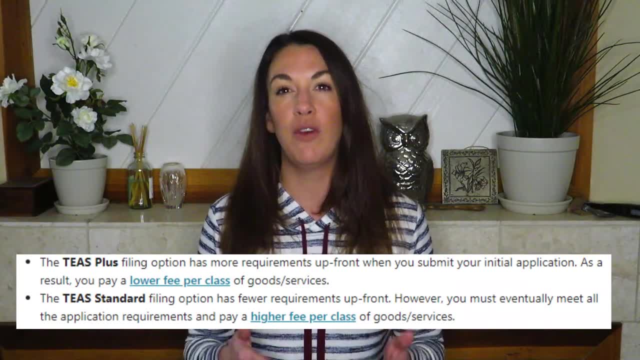 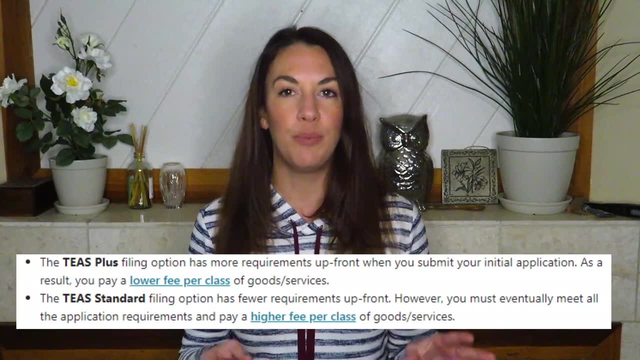 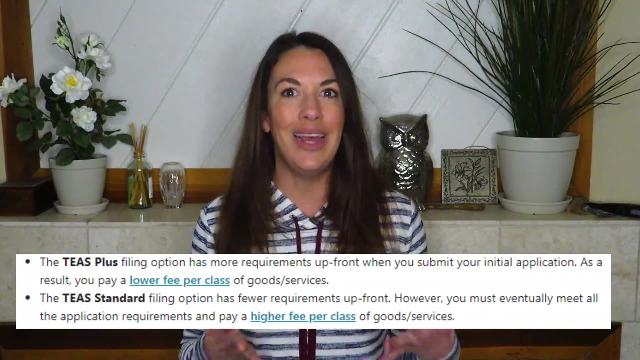 As the USPTO explains it, TEAS Plus has more requirements up front but a lower filing fee, And TEAS Standard has fewer requirements up front and a higher fee, Though in the end, the requirements for registration are exactly the same regardless of the application you use. So don't let the fewer requirements up front thing fool you. So the first major difference between the two is the filing fee. TEAS Plus is $250 per class of goods and services and TEAS Standard is $350 per class of goods or services. 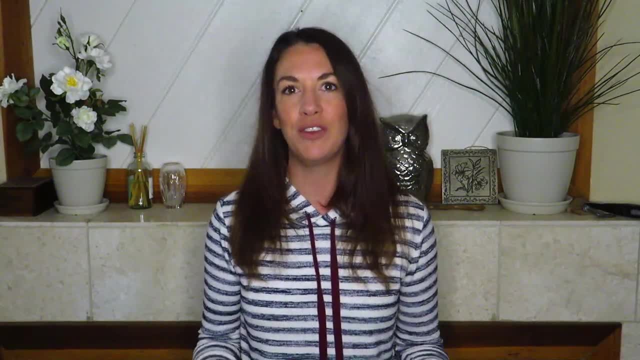 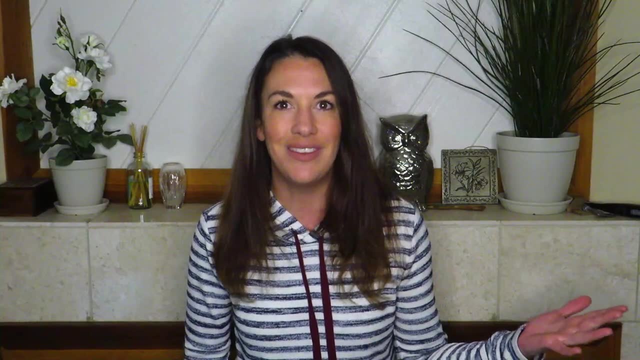 Obviously, $250 is better than $350, so most of us are going to want to stick with a TEAS Plus application if we're trying to keep our costs low. But, as the USPTO stated, TEAS Plus has more requirements up front compared to TEAS Standard. 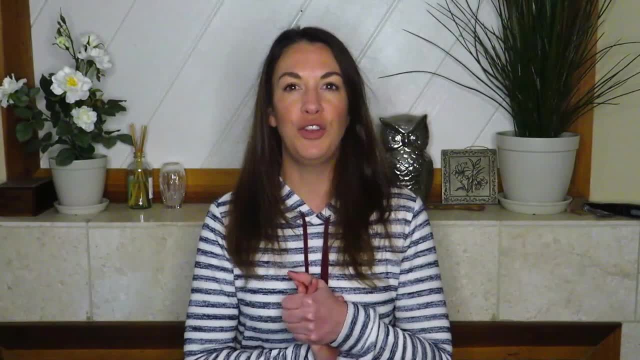 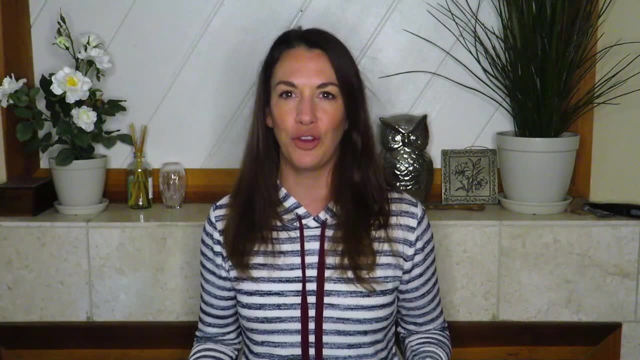 So let's talk about those requirements. The first has to do with when you pay the filing fee. If you're applying to register your trademark in more than one class of goods or services, all of those fees need to be paid when you submit the TEAS Plus application. With the Standard application, though, you only need to pay for one class when you file the application. The other fees, that there are any, will be due later on in the process. The second requirement has to do with how you identify the goods and services in your application. 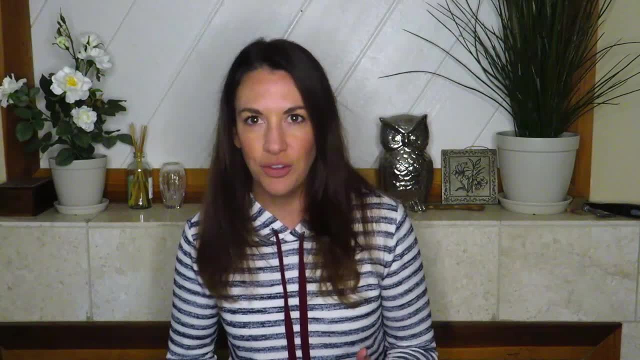 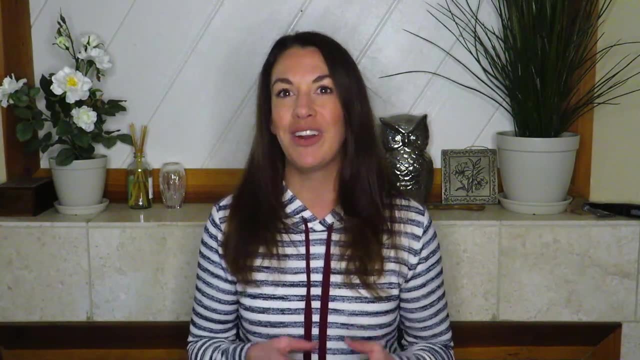 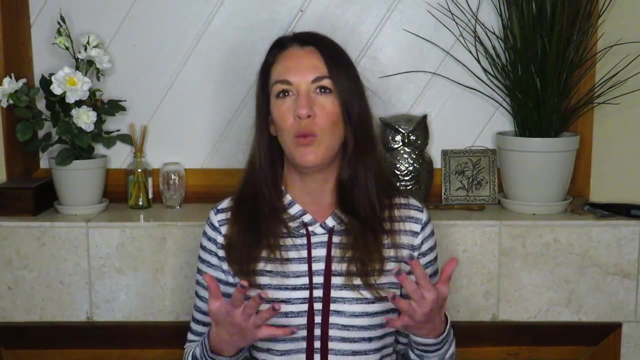 A little background real quick. When you apply to register a trademark, you have to specify the goods or services with which the trademark will be used. There are 45 different classes of goods and services and tons and tons of different categories or descriptions of goods and services within each class. As I mentioned earlier, the USPTO filing fees are per class. If you offer multiple types of goods or services that all fall under the same class, you can include all of those and only pay the filing fee for one class. But if your goods or services fall under multiple different classes, then there will be additional filing fees for those classes. 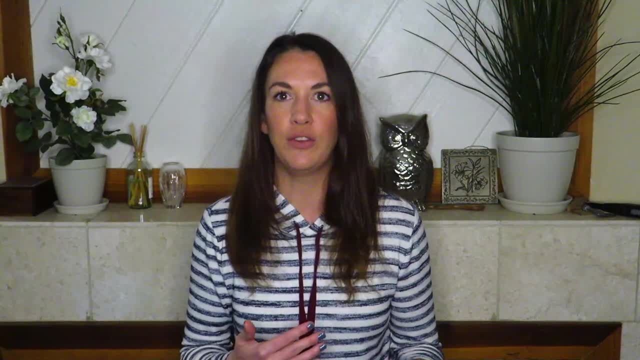 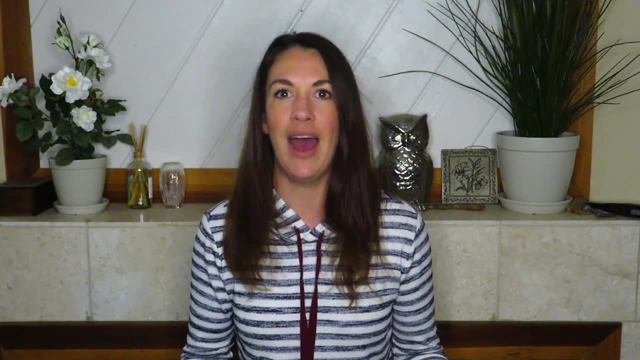 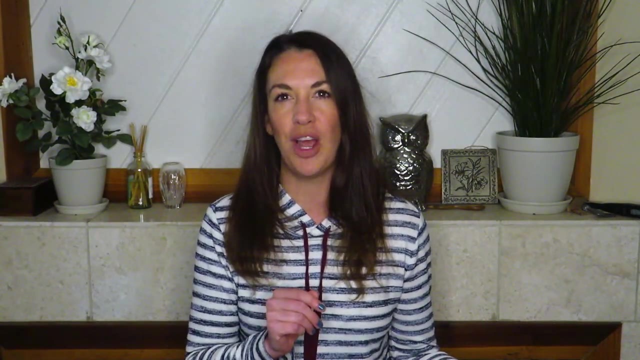 Okay, so back to the requirements for identifying goods and services. on your application, The USPTO has this thing called the Trademark Identification Manual. that has a huge list of goods and services. I'll link to the Trademark ID Manual in the description so you guys can check that out. 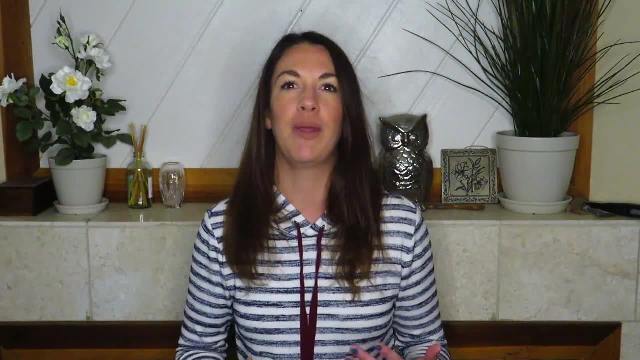 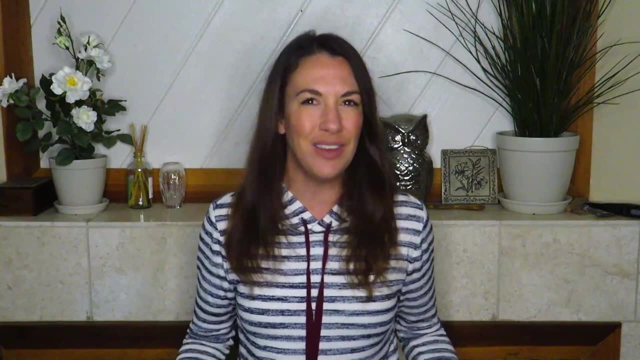 In order to use the TEAS Plus application and benefit from that lower filing fee, you have to select your goods and service listings from that Trademark ID Manual. This isn't going to be a problem for most of us. The Trademark ID Manual has a lot. 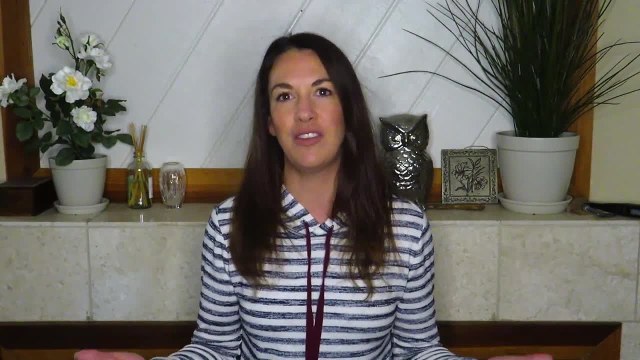 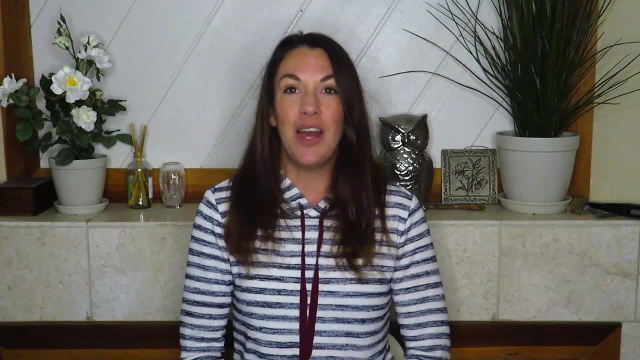 I'm talking thousands and thousands of different goods and services descriptions that you can choose from, and chances are there will be at least one in there that applies to you, But sometimes there aren't, Like if we're dealing with a brand new type of business. 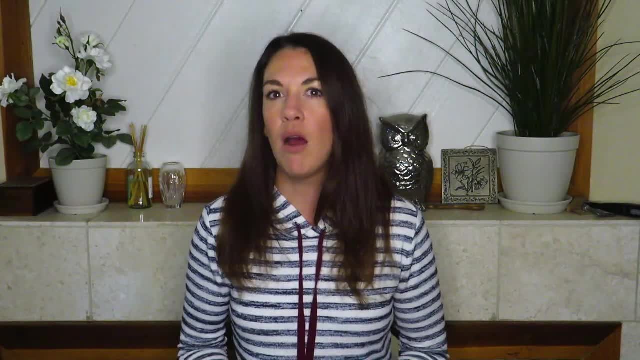 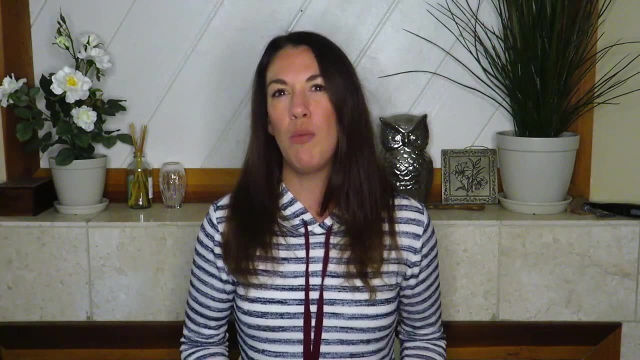 something that's never been done before. there may not already be a description in the Trademark ID Manual that really fits with our goods or services. Sometimes we need to be more creative and come up with our own brand new description for the goods and services. 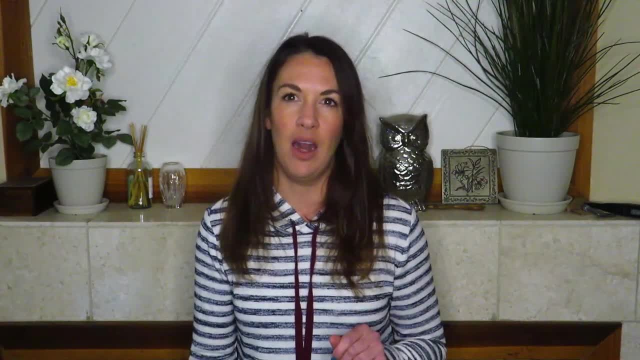 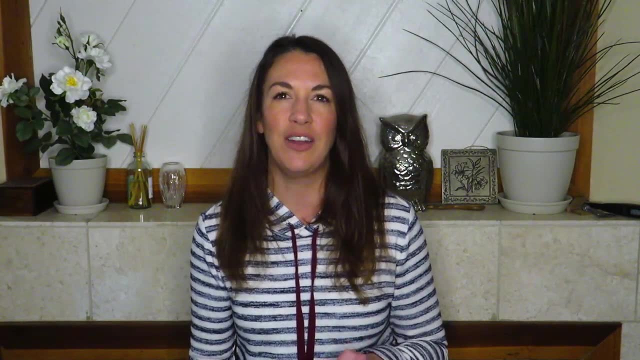 And that's where TEAS Standard comes in. Unlike TEAS Plus, where you have to pick from the Trademark ID Manual, TEAS Standard allows you to enter your own description for the goods and services under which you want your trademark to be written. 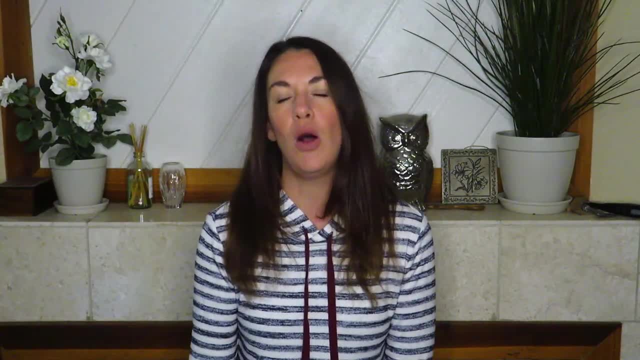 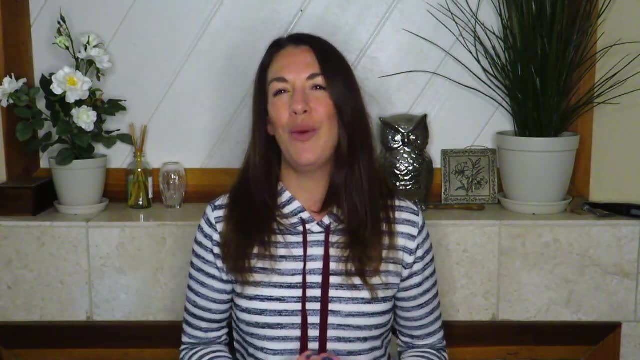 By the way, that's why the filing fees are not all due up front with TEAS Standard. We- meaning Trademark applicants and Trademark attorneys- don't always know exactly which of the 45 classes would be appropriate for the goods and services. 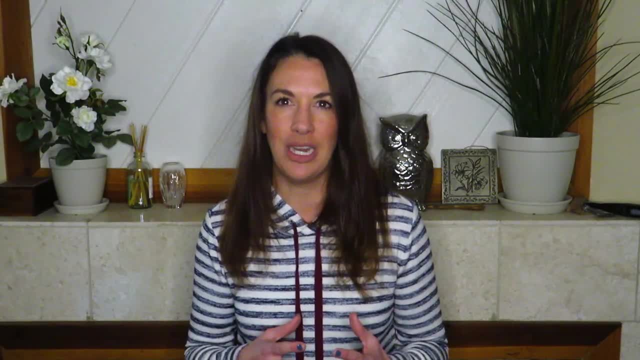 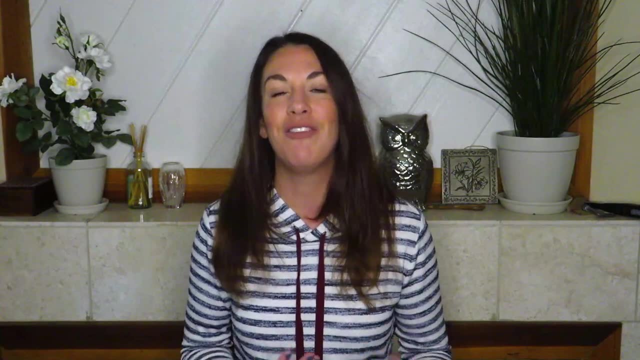 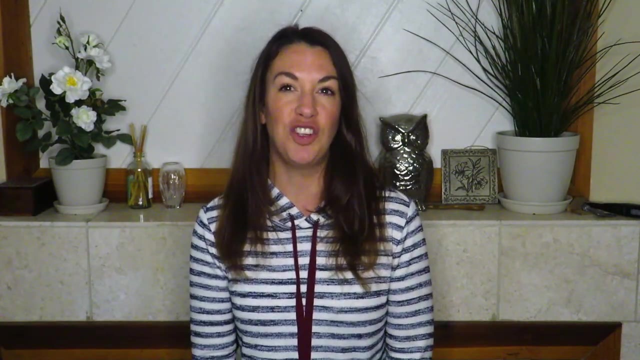 So we're allowed to leave the class number out of the application initially and basically let the USPTO tell us which classes are appropriate And then we can later pay the additional filing fees if needed. The third extra requirement for the TEAS Plus application: 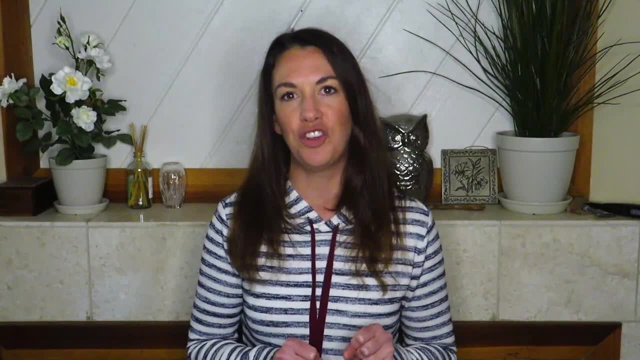 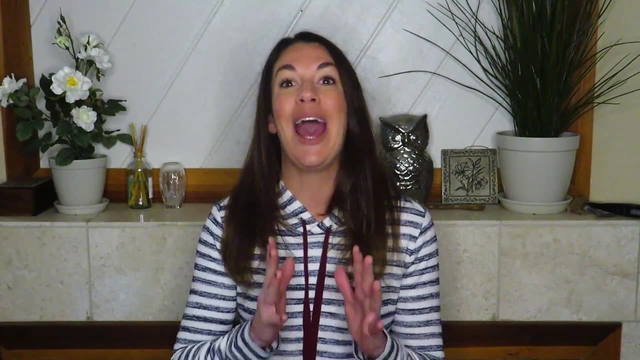 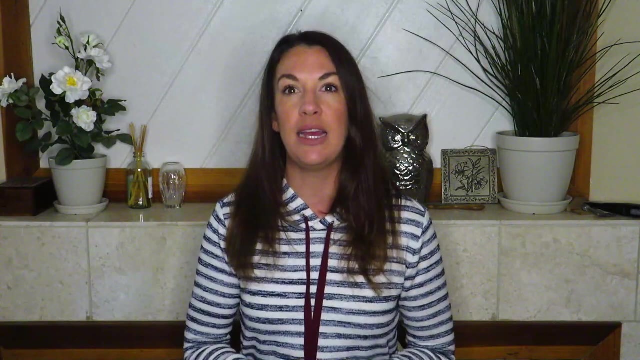 has to do with the additional statements portion of the Trademark application. There's a section on the application that asks about additional statements With TEAS Plus. we have to indicate on the application if those additional statements apply to our trademark Specifically with the TEAS Plus application. we have to address. 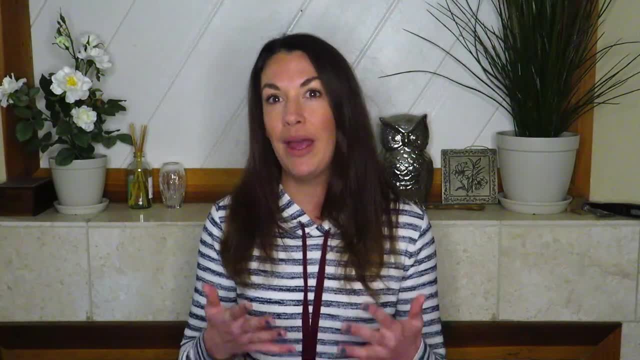 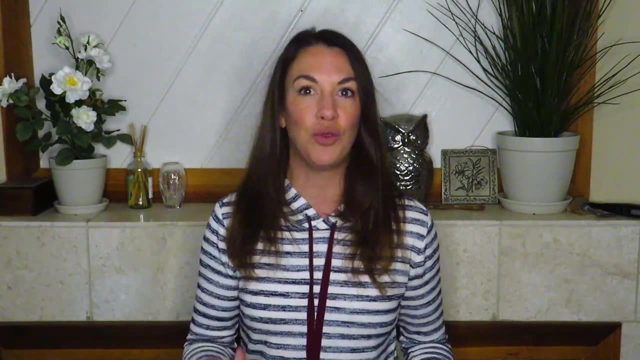 if the same trademark has already been registered with the USPTO by you, but the owner name in the prior registration is not the same as in the new application. if the trademark has color. if the trademark includes a design or stylized font. 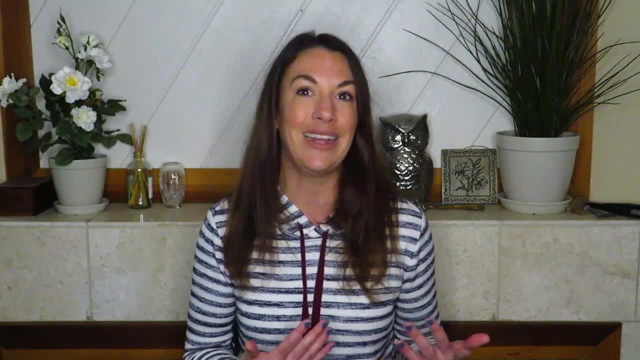 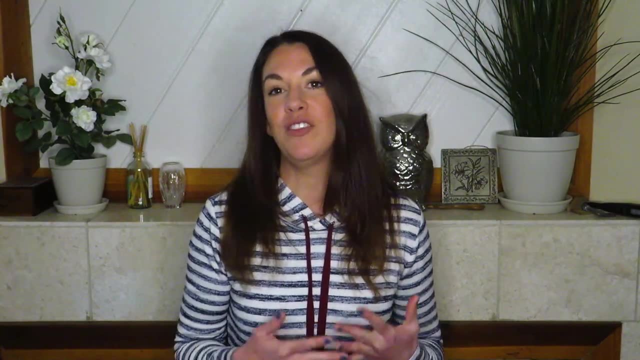 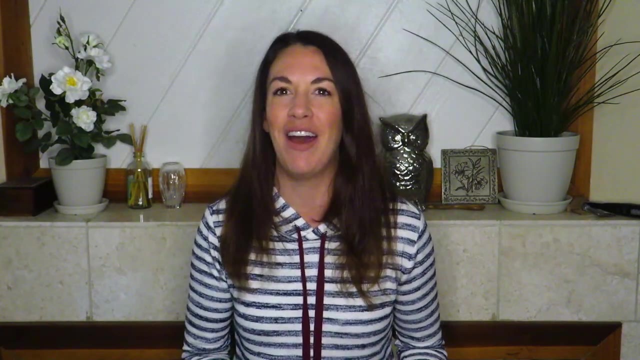 if it includes non-English words or non-Latin characters. if the trademark includes a name or portrait of a living individual. and if the trademark is currently in use and the applicant needs to limit use to specific geographic area and identify the other concurrent users. 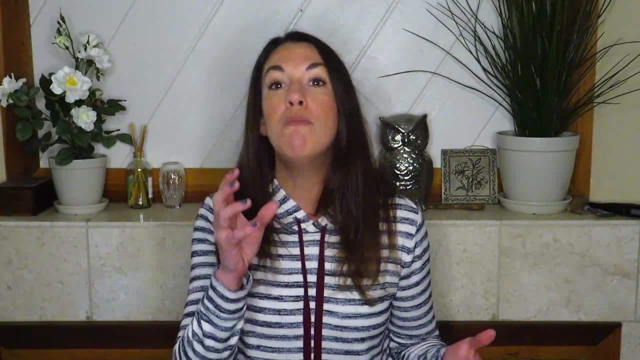 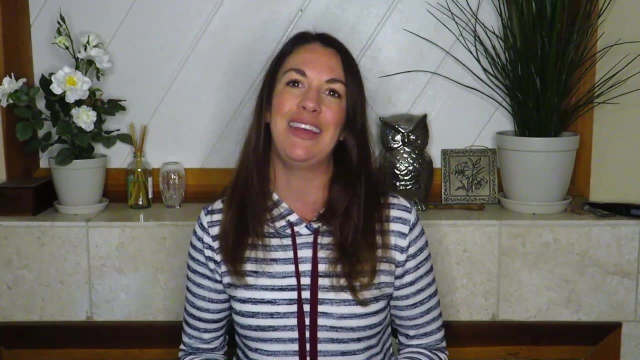 So if any of those circumstances apply to your trademark, you must indicate that on the additional statements section of the application. if you want to benefit from that lower fee of the TEAS Plus application, This is super important because the USPTO is going to charge you additional fees. 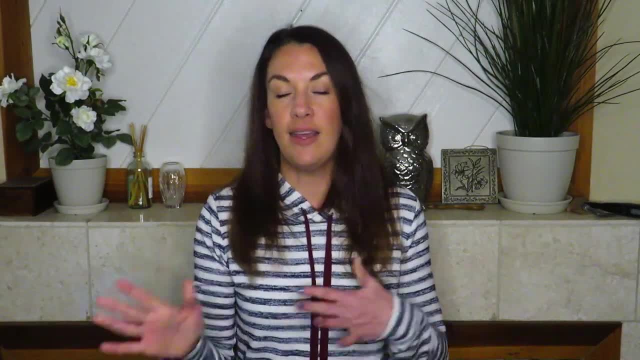 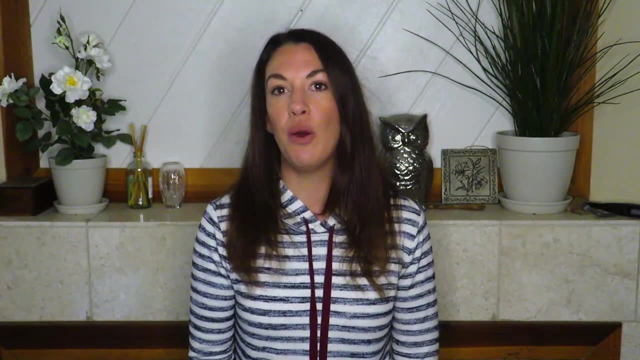 if you fail to do so when you should have. The TEAS Standard application, on the other hand, doesn't have that requirement. You will still need to tell the USPTO if any of those additional statements apply to your trademark, but you can do so after the application has been submitted. 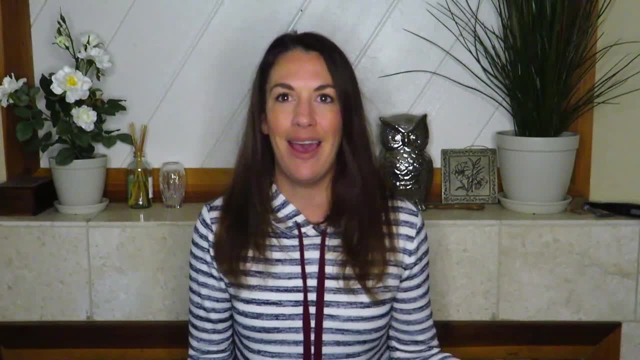 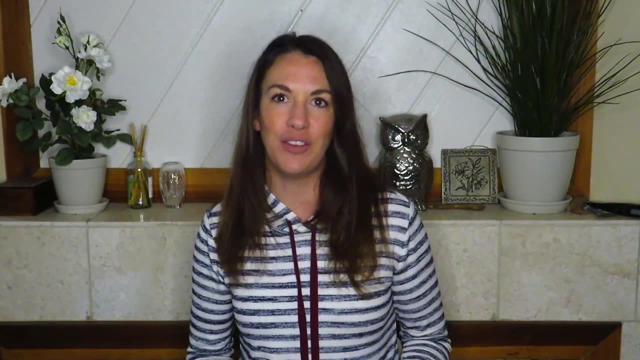 So, to summarize, the main differences between TEAS Plus and TEAS Standard are: number one, the filing fees. number two, how we select the goods and services for our trademark. and number three, when we need to indicate if any additional statements apply to our trademark. In the end, the requirements to get a registered trademark with the USPTO are exactly the same, regardless of the type of application you use. Using one application over the other isn't going to decrease your chances of getting rejected due to a likelihood of confusion, for example. 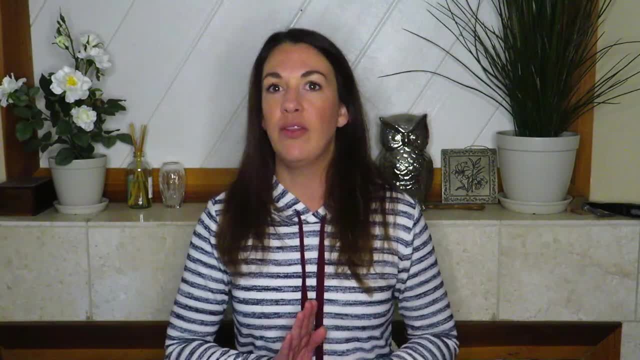 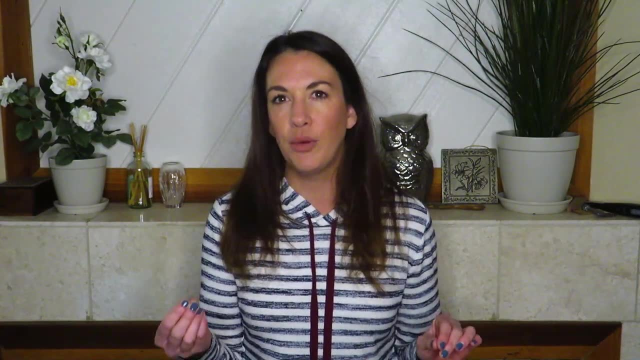 If we're trying to keep our costs and filing fees low, then the TEAS Plus application is going to be the best and most appropriate option for most of us. The most common reason for using the TEAS Standard application is if we need to go outside of the USPTO. 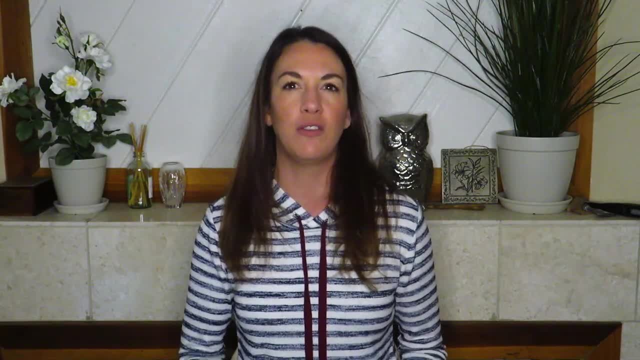 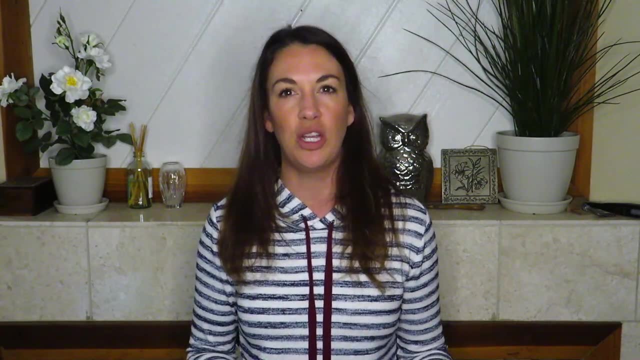 We're not going to be able to access the USPTO's trademark ID manual for our goods and services descriptions. But with TEAS Plus it's important to pay close attention to those additional statements on the application to make sure we don't miss any important detail. that might result in additional filing fees. That's why it's always best to work with an experienced trademark attorney if you are trying to get a registered trademark with the USPTO. Sure, a lawyer is going to cost more money, but it will help you increase your chances of getting the trademark registered. 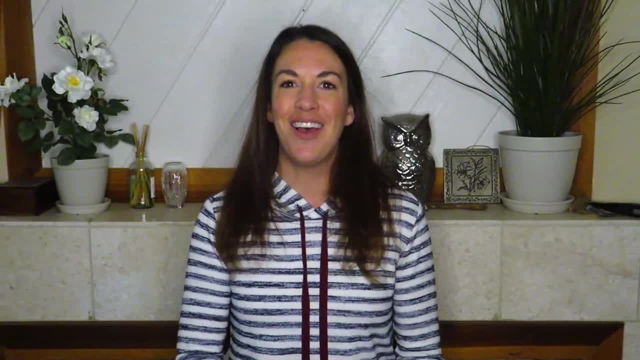 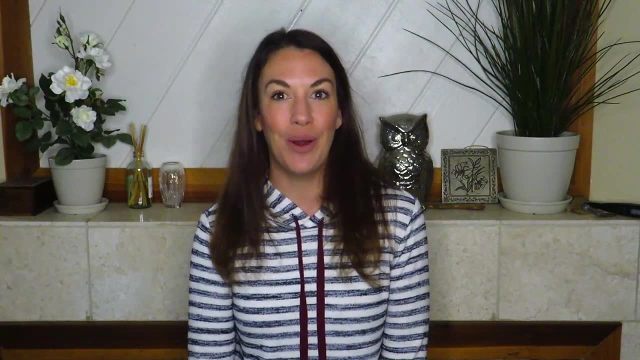 and prevent costly mistakes on the application itself. That's all for this episode. folks Drop a comment below. Let me know what you think. If you need help getting a registered trademark for your business, check out Brand Bombshell, my signature all-inclusive trademark registration package. 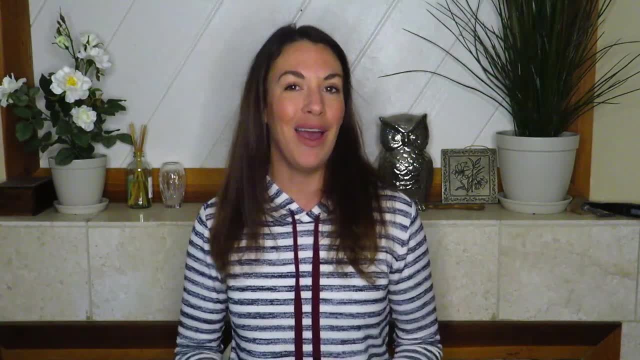 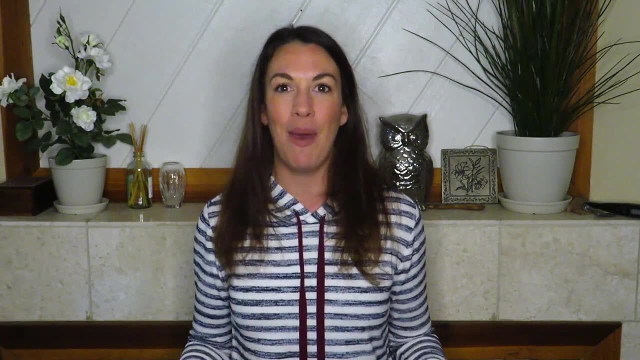 Or if you're on a tight budget and looking to DIY your trademark application, then check out Brandish, my on-demand online course that teaches you step-by-step how to prepare for, complete and submit a trademark application with the USPTO without a lawyer.